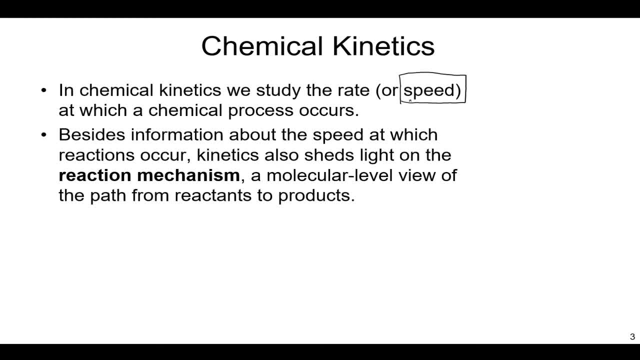 that reaction. But this is actually not the most important aspect of kinetics. The application that's actually more important is that it tells you something about the reaction mechanism, And this is really key in chemistry. This is what is allows us to use chemistry to actually do. 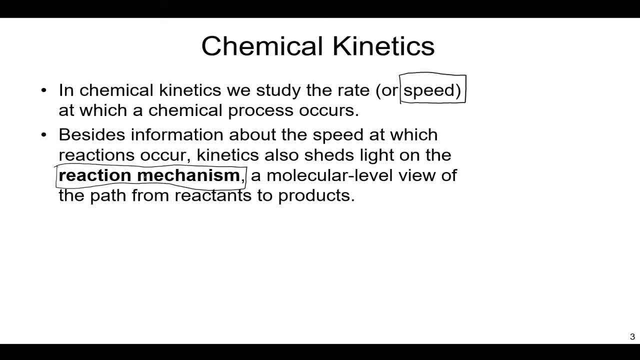 something useful like create a new catalyst for promoting some reaction, or inventing a new drug that blocks or inhibits some other mechanism in your body, And so mechanism is really the whole point of this, And as an example let's look at a quick reaction here of NO2 in the gas phase. 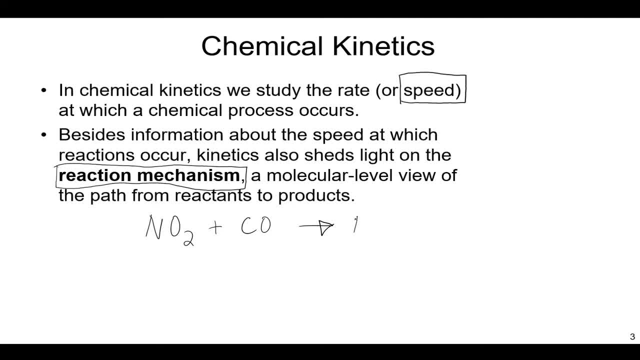 plus carbon monoxide, And this can make NO nitric oxide plus carbon dioxide, And so this is the overall reaction, right? When we write chemical reactions like this, we usually write reactants and products: reactants on the left, products on the right. Okay, and this is sort of the start, and 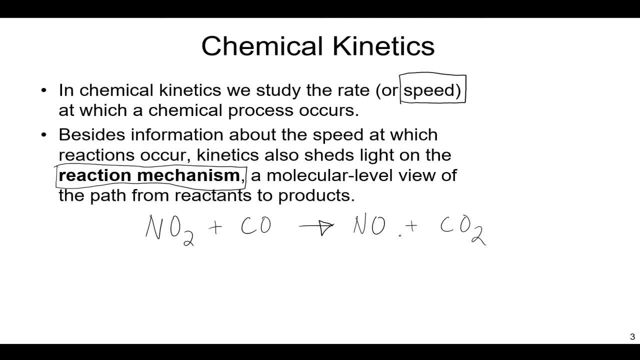 finish of the reaction, But it doesn't tell us how the reaction occurs. The mechanism tells us something about the molecular level view from reactants to products, And so if I asked you to come up with a mechanism, you might say: Okay, well, you know this molecule, this is on the gas. 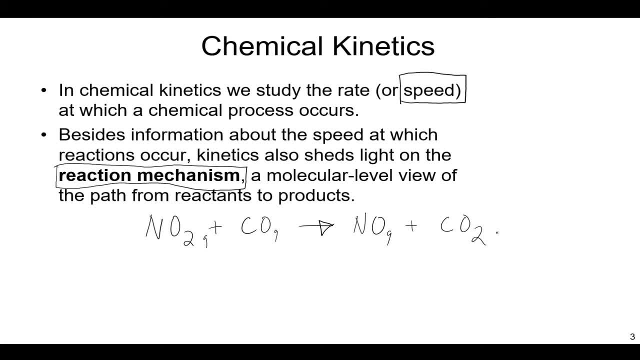 phase. although I haven't labeled it here, these are all gases, And so you might say: Okay, well, CO in the gas phase simply bumps into NO2 and steals one of its oxygens, adding it to make CO2, right, that seems very reasonable that this two molecules would bump together and an oxygen would 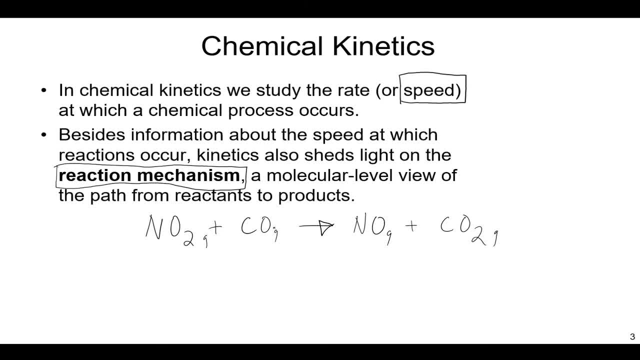 get transferred. But that's not what happens. You have to use chemical kinetics- as we'll see over the next series of lecture, to actually figure out what the mechanism is And the mechanism for this reaction is, although it's that overall, it happens in two steps, And the first step is actually this NO2 molecule has to. 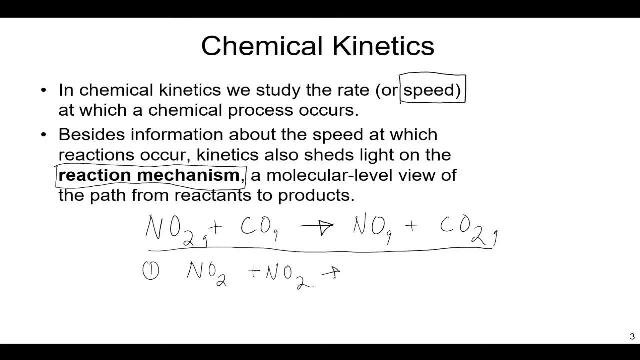 bump into another NO2 molecule first, And so what really happens here is the oxygen transfers from one NO2 to the other, forming NO3 and NO. Notice. this product right here is shown right here. So the first step creates one of the products. 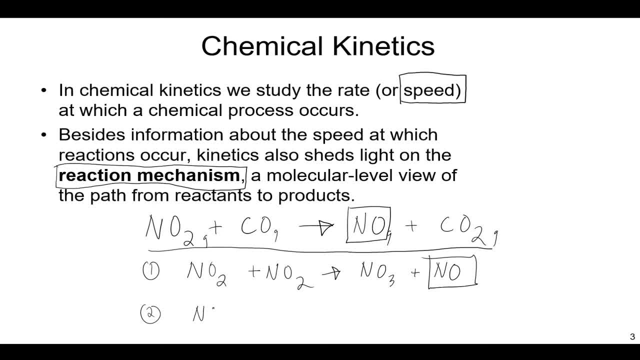 then, in step two, this NO3 that you've made in step one is what bumps into carbon monoxide, And that's where another oxygen gets transferred, And there you're making an NO2 and a CO2.. Right, and so this second product, CO2, comes from this second reaction here. Now, overall, this NO3 you made in 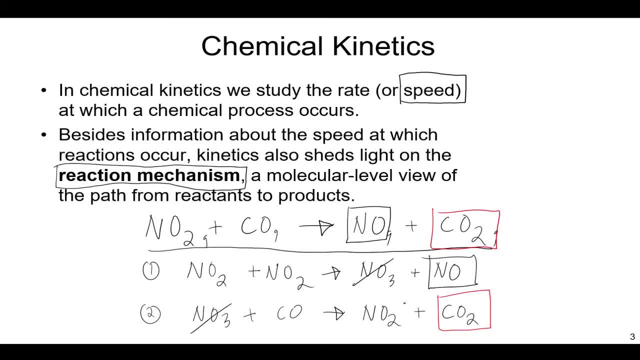 step one cancels with the NO3 made here and NO2 you make in the end cancels with the NO2 here. So yes, overall it's NO2 plus CO, making NO plus CO2, but that's quite different than at first look. 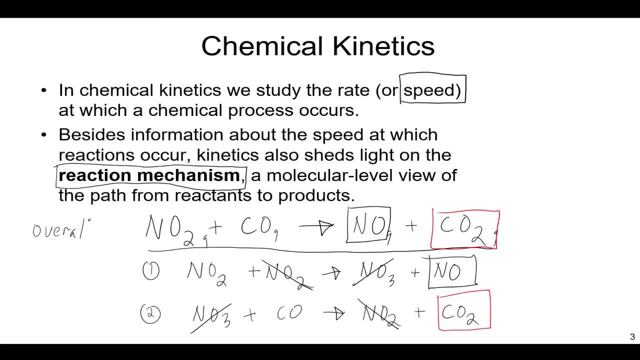 what the overall reaction might suggest as a mechanism, And so this is about as simple as it gets for a reaction mechanism. You can imagine more complex chemistry, like what takes place in the human body, is a lot more complex, But it's always about using kinetic theory, which depends. 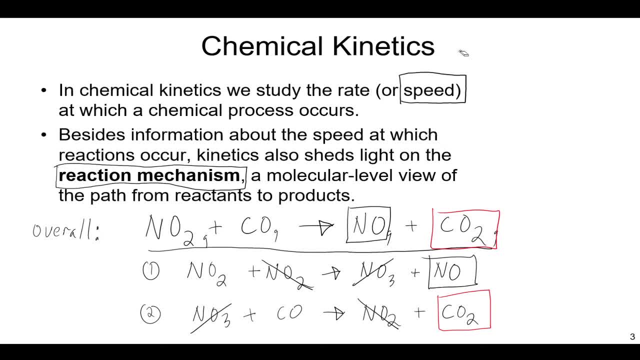 on measuring speeds and rates of reactions to figure out the underlying mechanism. Today we're going to mostly focus on the first bullet point and future lectures on kinetics will build up to understanding mechanisms. but they're really experimentally derived from these rate measurements. 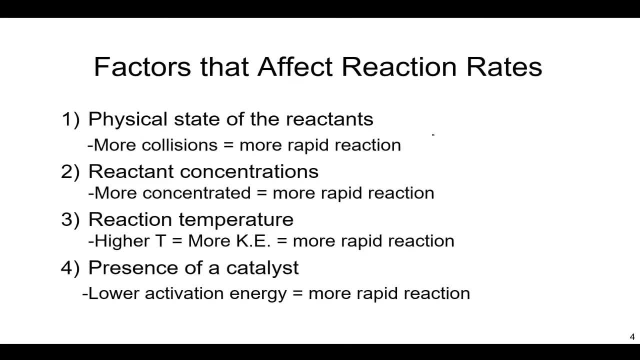 and speed measurements. So that's really where we're going to start. The factors that affect these speeds or reaction rates are shown here. Physical state of the reactants definitely matters. You can imagine one solid reacting with another. solid is probably not very fast. 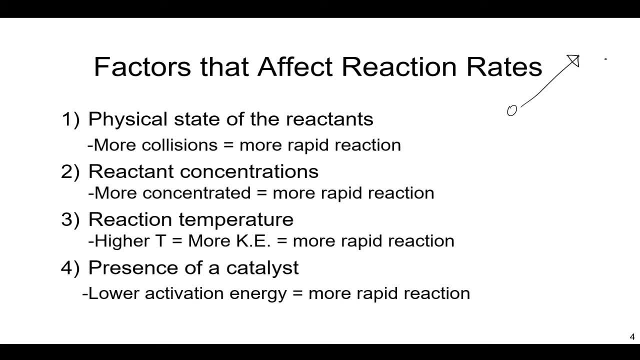 But a gas that is colliding around might bump into another gas molecule, whereas a solid might not bump into another solid. Okay, so the more collisions you have, the more rapid reaction. right, So the state of the matter matters To be redundant gas faster than liquid. 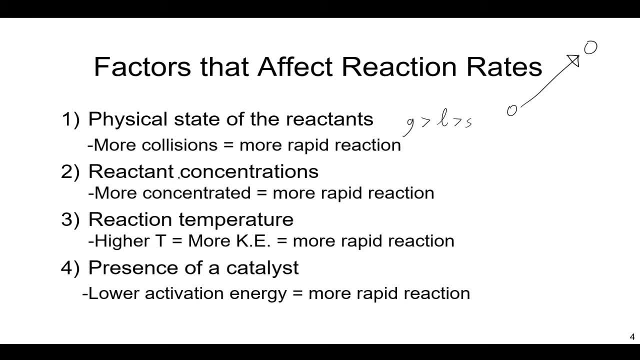 faster than solid usually. The second factor that matters is concentrations. This seems to make sense. The more things you have around, the more reactants you have around, the more times they're going to bump into each other right, And the more rapid that reaction will become. 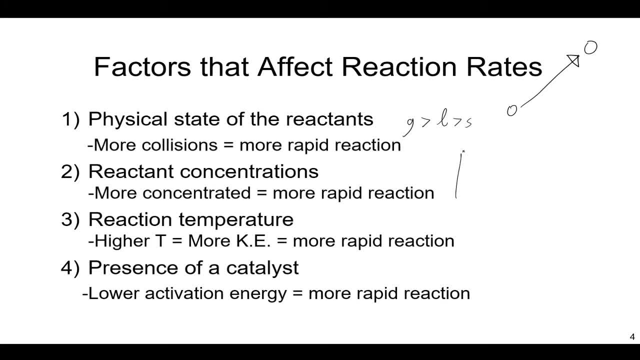 So concentration is definitely going to matter. You know, if in this volume you have two gas molecules, it's going to take a while for them to bounce into each other and find each other right. But if the concentration is much higher and there's 18, 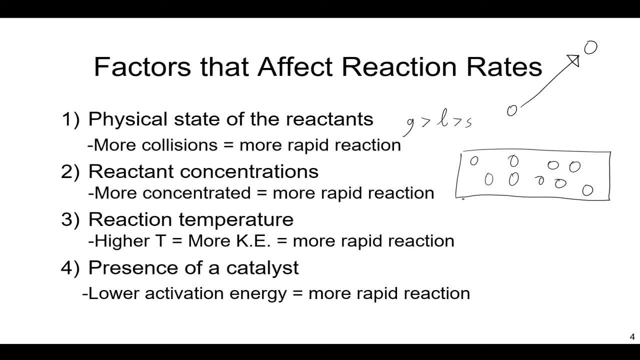 molecules- or I don't feel like drawing 18, let's say nine molecules, well, obviously the reaction can proceed much more rapidly. The other thing that matters is reaction temperature. This suggests the higher the temperature, the more rapid the reaction. So if you still have two molecules, that 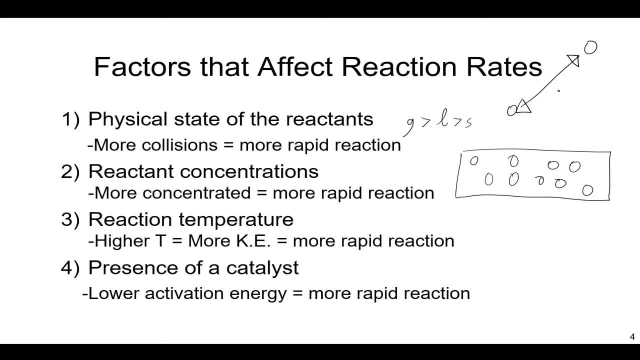 must meet up for a reaction to occur. well, if they have more energy, they're zipping about the room faster, they're more likely to meet up, And if they have more energy they're more likely to, but they're also more likely to overcome some activation energy Okay, so temperature actually. 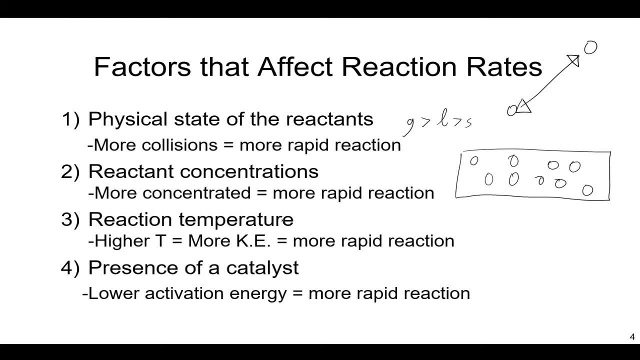 matters twofold: It supplies more collisional opportunities, but it also has a higher energy per collision which might be required for the reaction to occur. And the fourth factor that matters here is the presence of a catalyst, which we'll talk about in a future lecture. But this 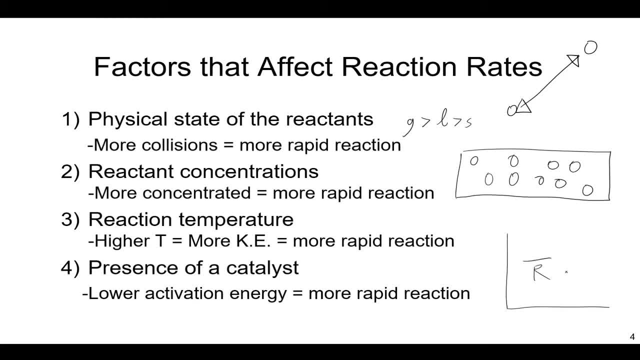 basically changes on these energy diagrams from reactants to products. it really reduces the amount of activation energy needed here to get from reactants To products right. a has to get over this hump. to get to be So those are sort of four factors. 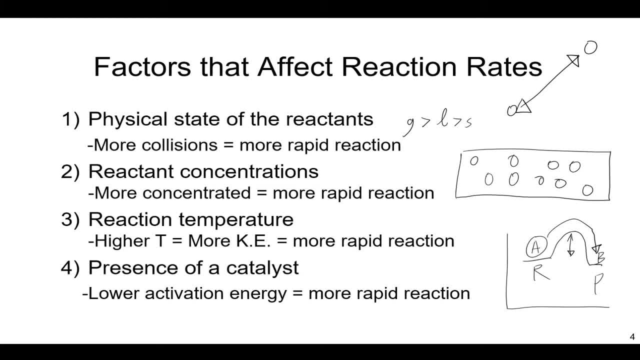 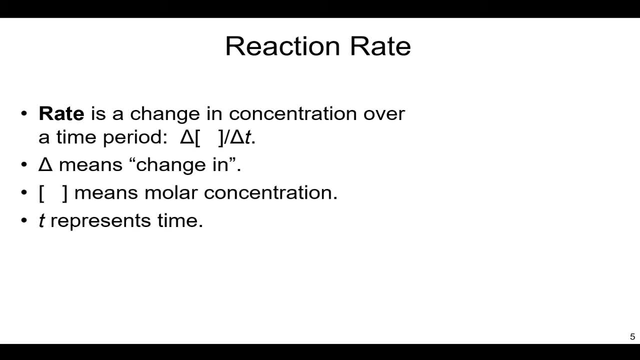 that affect reaction rates, as we're learning some of the things that matter for the speed of chemical reactions. Now the bulk of today's lecture, and certainly going forward with our other kinetics lectures, is going to be determined by reaction rates, which are really just rates of. 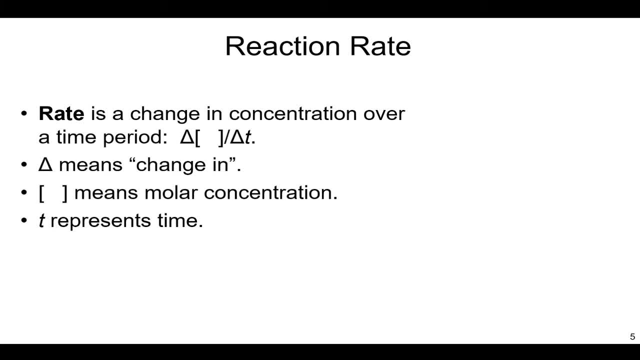 change. So this is really fundamental math. we're just applying to chemistry here a rate of change being a change in concentration over a change in time period, right? So our delta here is, you know, means change in some final minus initial, right we're. 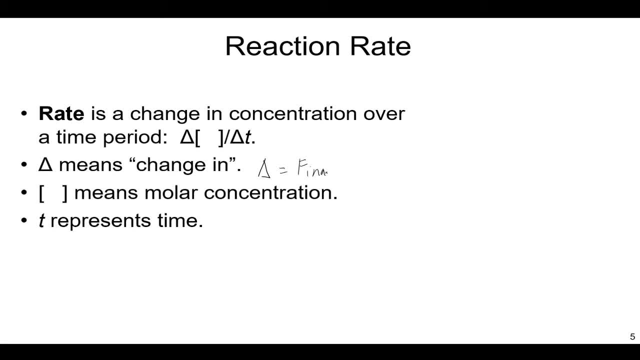 going to take final concentration minus initial concentration or final time minus initial time and these measurements that we're making in the laboratory. the concentration here is our molar concentration. sometimes you'll see like partial pressures of gases, but most of chemistry. 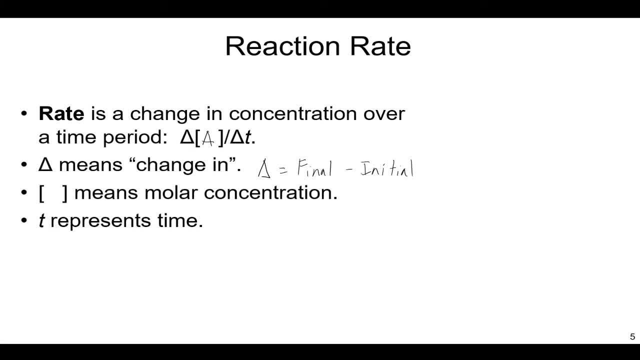 especially that we discuss in this lecture is going to be about concentrations in the liquid phase, aqueous phase moles per liter. the T here represents time. So let's think about some really basic chemical reaction. right, some reaction A turns into B- pretty exciting, I know. 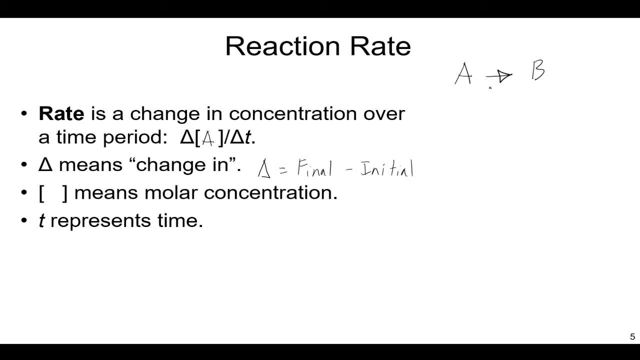 but it illustrates the point of how you're going to calculate a rate: A turning into B, the rate of this reaction. okay, we can think about this as a rate of change. we're going to calculate a rate of change and we're going to calculate a rate of change. 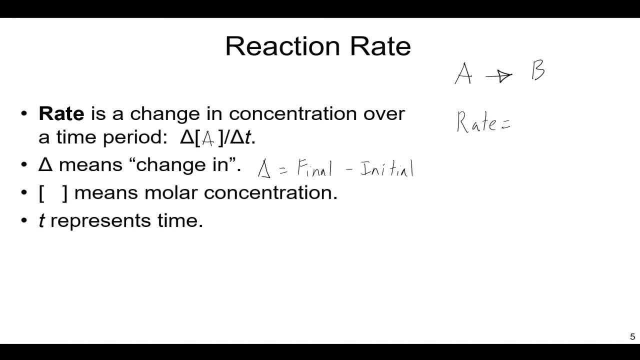 rate as being this change, and here the real change that we want is the product, what is being formed. okay, so this is going to be a change in b concentration over a change in time and sometimes when you get into calculus, you might see this as these derivatives: db, dt. 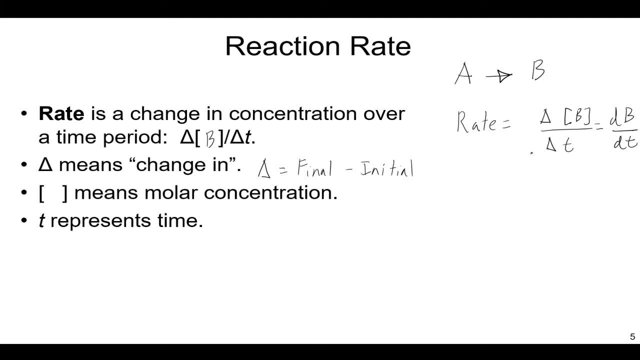 okay, for now we'll stick to this sort of delta symbol. now imagine we start this reaction at time zero and we monitor the concentration of b, and maybe we set up our experiment so we start with only a. so at time zero, when we start the clock, there is no b yet, and a minute later, 60 seconds. 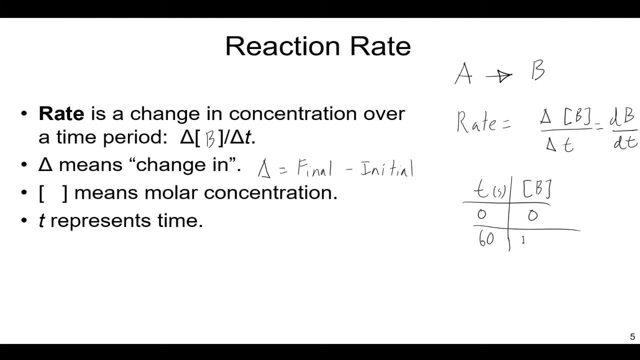 later we measure the concentration of b, and 1.38 molar is the concentration of b and you can measure this a variety of ways. you can measure it by taking the concentration of b and taking the values, maybe spectroscopically, where you're shining light at the solution and monitoring some. 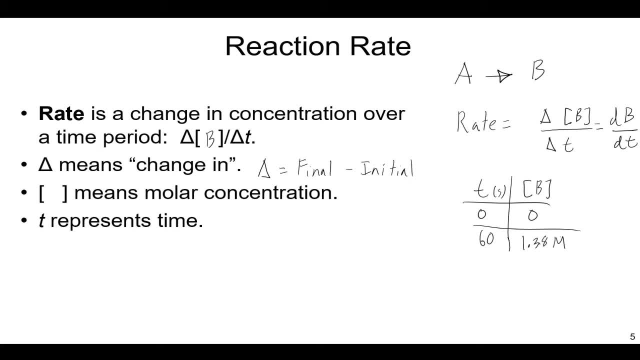 absorption band, for example, regardless. here's the data points i collect. it's really this simple. the rate then is just the change in concentration of b- b final minus b initial over time- final minus time initial- and so my overall rate here would be something like 0.023. make sure you do better than. 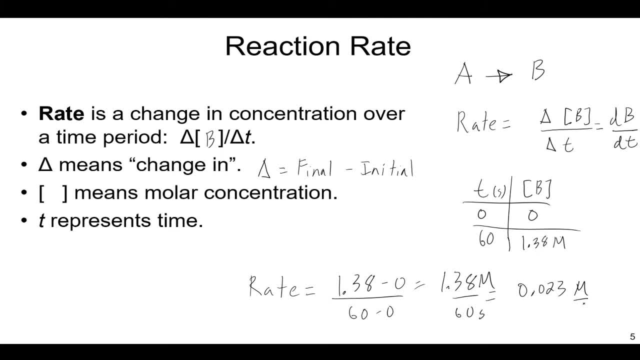 me and keep track of your units. 0.023 molarity per second. okay, and this rate, since it's defined as this concentration per time, is always going to have these units here. now, instead of seeing how b is produced, we could also see, so here is how b is produced: delta b over delta t. 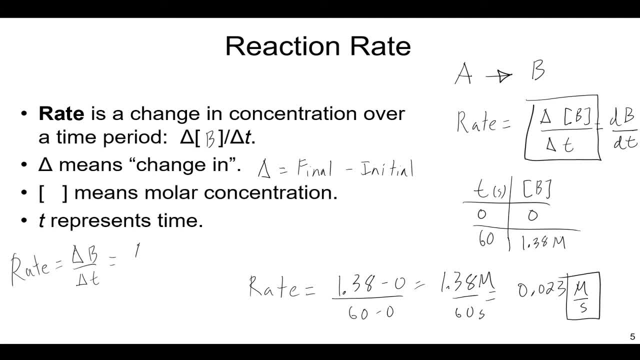 maybe you can then just you can take a look at this here, but you don't remember that. here is this a double index and this is a root B. we could also observe how a is disappearing right change in a. i should probably put this in brackets over change in time, but i want to make one. 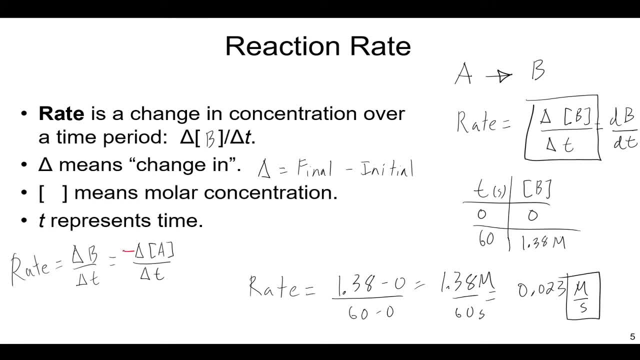 important point here is that if it's a reactant, put a negative sign out here. by convention the rates are positive for making a product okay and the rate should still be positive for where we're considering a reactant. but initial our delta a is going to give us a negative number, so we put this negative sign out front to. 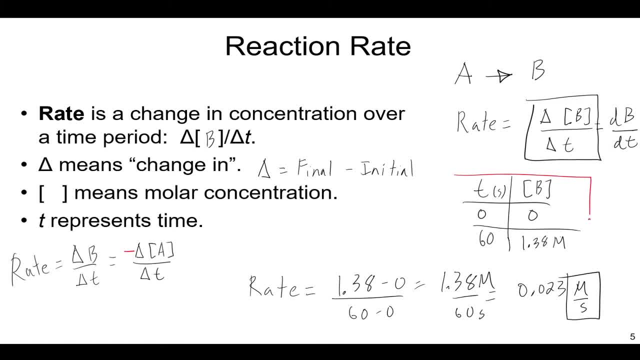 combat that. so in your calculations of rates, if you're doing it like we just did here, if it's a product, don't worry about the negative sign. but if it's a reactant, like a here, then we're going to include this negative sign here in our calculations. so rates usually indicate how. 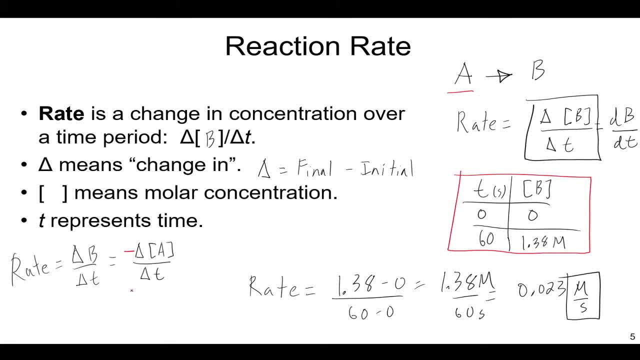 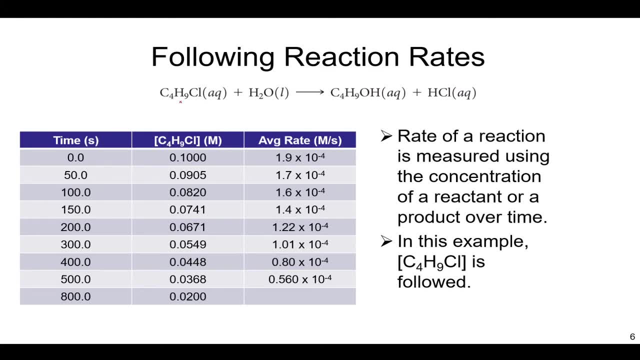 the product is appearing, but it also means how the reactant is disappearing. now let's look some actually add some actual tabulated data for this, and here we have c4h9cl and water that's making this hydroxide version of it with an acid hcl, and you know, we can start the clock at time zero, and 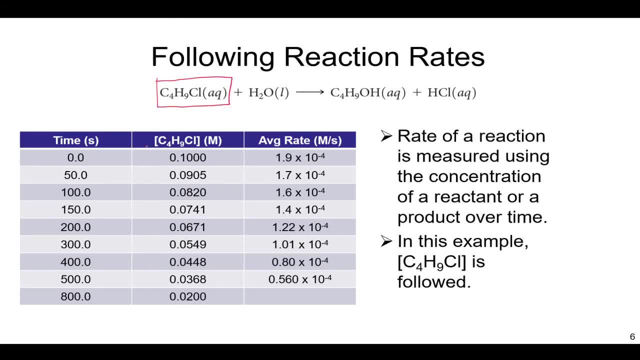 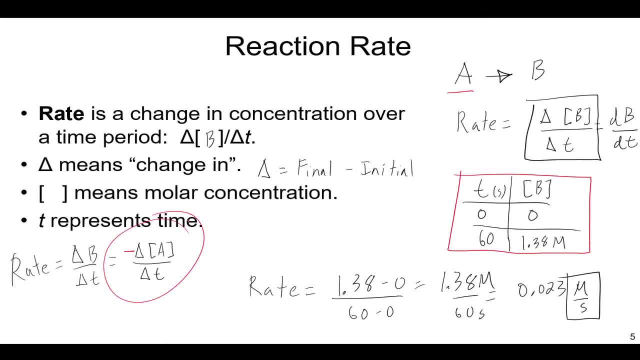 we can monitor the disappearance of this right and we can calculate the rate from any subset of data here- between 0 and 800 seconds, or 0 and 50, or 0 and 100- just by taking the corresponding data and doing the calculation that we just showed back here. 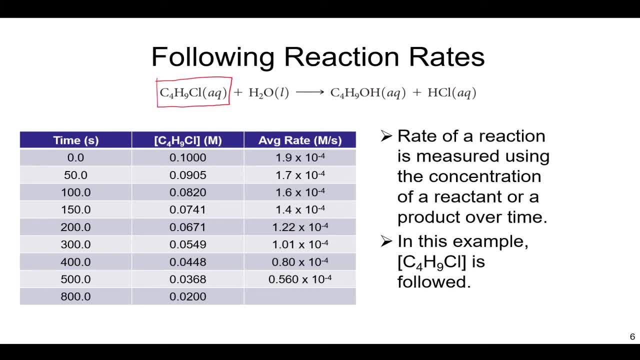 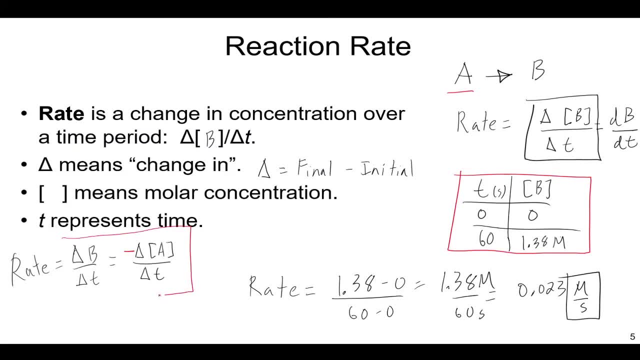 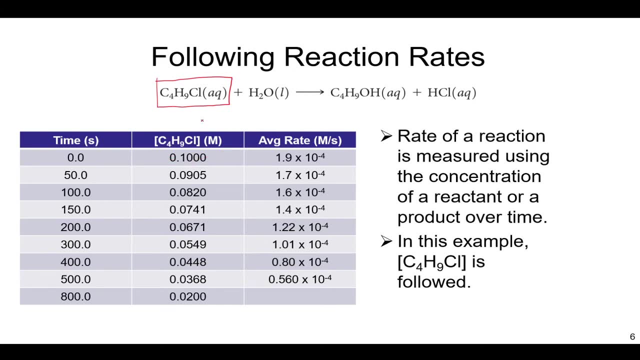 so the rate of this reaction really means you only have to monitor one of these components. the rate is always going to be equivalent, right? so these two things are related. i don't have to measure both a and b, i only have to measure one of them. that's why we can only measure one thing here: this reactant, and we can figure out the rate of the. 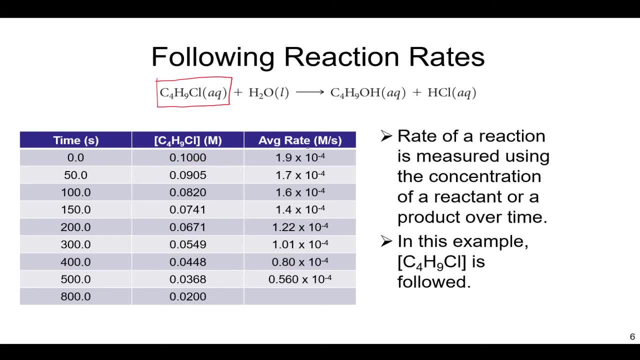 overall reaction because it's all related. so to get a number like this here, all they've done is calculated. well, what is the negative change in this is from 50 relative to zero. okay, so this rate comes from these two, just like this rate would come from this one and this one. so the average rate here is actually looking at any two. 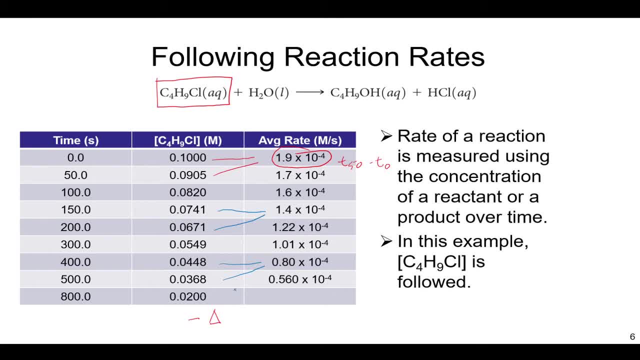 successive measurements. you don't have to do that. you could do zero relative to 800, but just in this table that's where these numbers come from. so let's look at this first number just to make sure we can calculate it out correctly. this average rate 1.9 times 10 to negative 4 should: 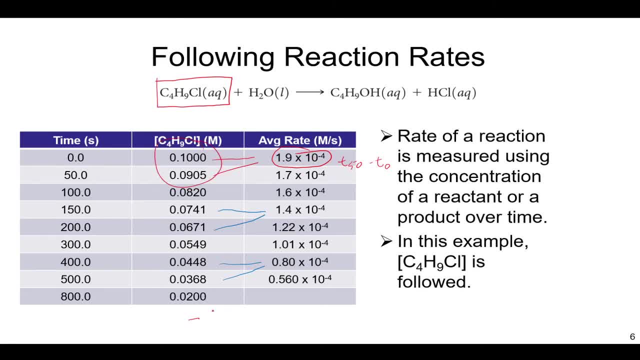 be the change in these concentrations. so final 0.0905 minus 0.1, divided by 50 minus zero, which is just 50, and that number, should this negative sign, will cancel out the negative sign you get from this subtraction to give you an overall. 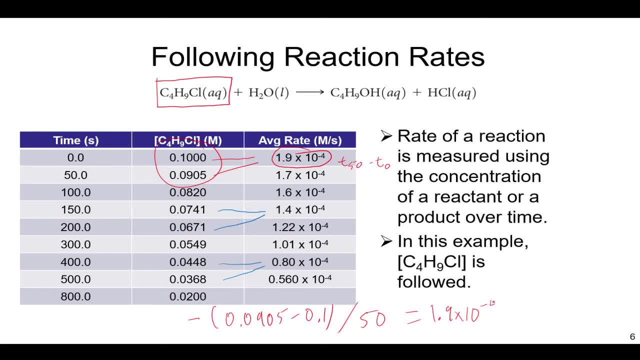 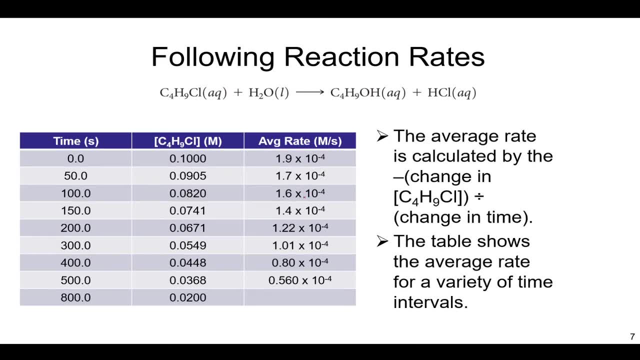 answer of 1.9 times 10 to the negative 4. okay, so this is just showing you how you calculate these successive average rate measurements. that's all this says right here, so we can watch this rate change over time. and this is what's tricky, and not always obvious from first glance, about these reactions, or any reaction right is. 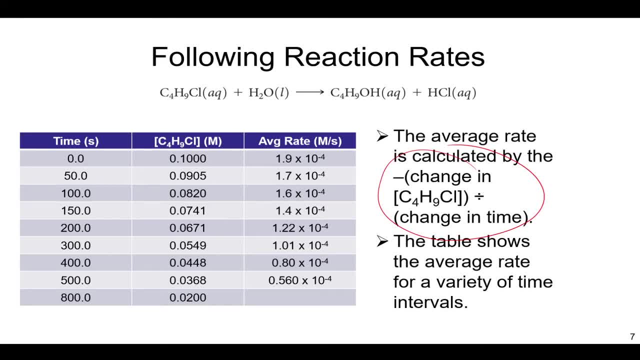 the rate that that process is occurring is changing over time and eventually this is a little bit early, but eventually we'll see how this leads to an equilibrium, when forward and reverse reactions end up being the same, because the forward reaction is slowing down and the reverse reaction is speeding up. but that's getting a little bit ahead of ourselves. 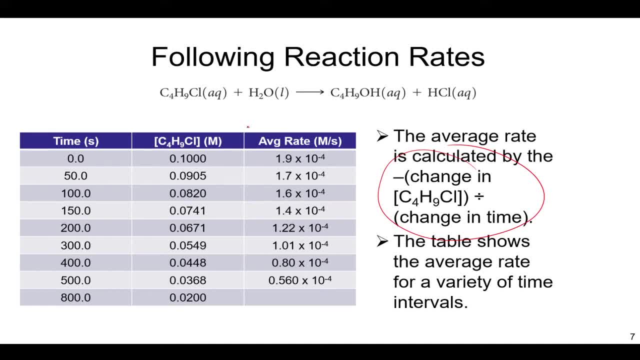 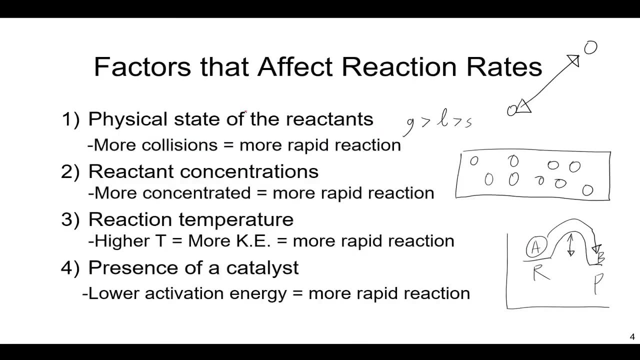 so the rate is decreasing with time. all of these, you see, are decreasing right, and that makes sense because if let's think conceptually, if the reaction has to happen by this molecule bumping into a water molecule, well let's go back and review what the rates depend on. rates 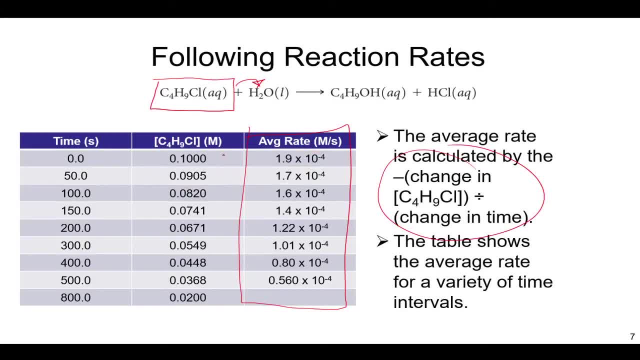 depend on concentrations. so as this reaction happens and there's less and less of this, well, there's less and less of it to meet up with water to make the product. so the rate is very slow here at the end because there's simply not a lot of that reactant left to react and in tables this: 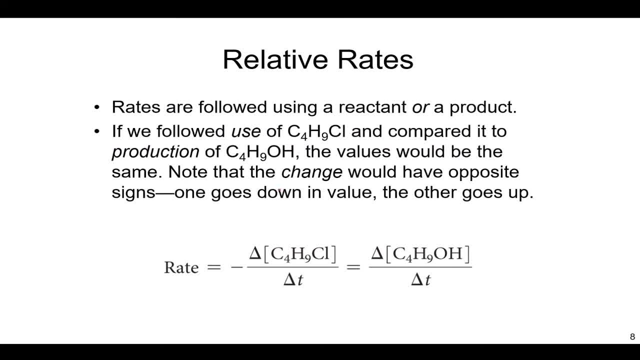 gets a little bit, uh, onerous to follow, uh, so it's much easier to graph these things. again. we can calculate it from this, which we were just doing, but this is going to be equivalent to the production of this product. so this was the reactant here. this is the product. you know, if one goes down, the other goes up and that's expected by. 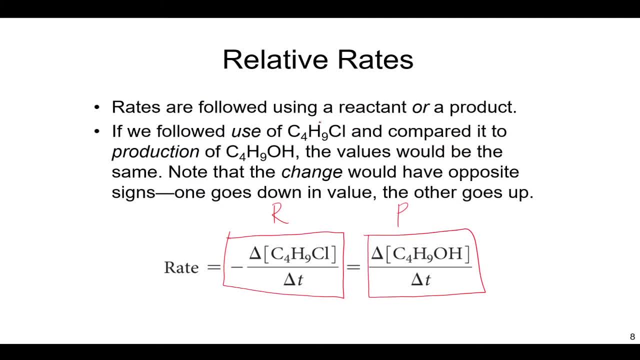 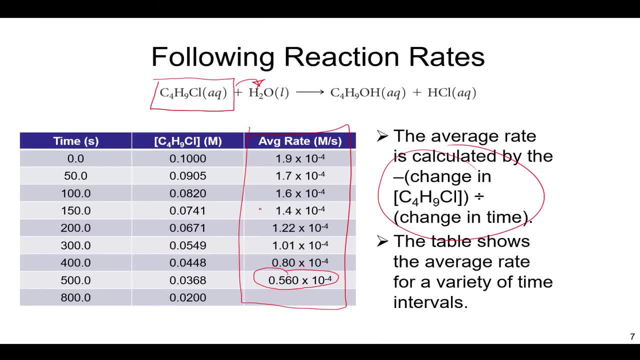 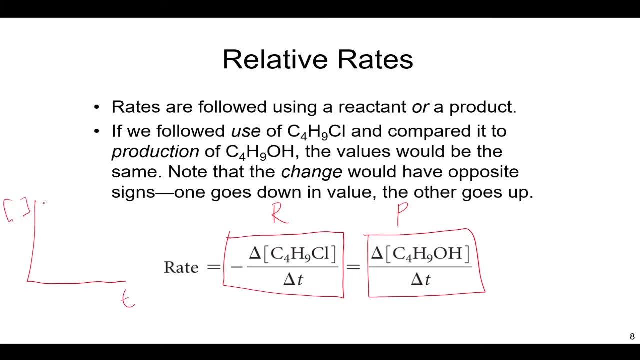 this relationship here in the chemical reaction. now, looking at this on a graph, we could plot this product. okay, so the reactant that we just looked at here, which is decreasing right on a graph, if this is our concentration versus time, well, that reactant is decreasing. if we wanted to plot. 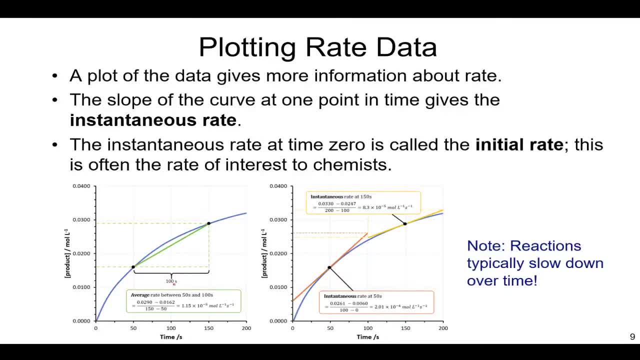 the product. well, the product would be increasing and looking like this- this blue graph on the left or the right here- and the plot is a lot better. it's more informative, it makes it easier for other science scientists to follow. so instead of giving the just the table we usually plot, 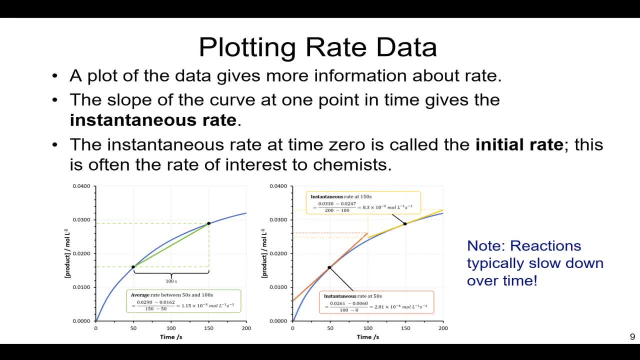 these things. now, the slope of the curve at any point gives us this instantaneous rate. so draw a the curve and that'll tell you sort of the instantaneous rate at that point. so there's an instantaneous rate, there's an instantaneous rate, here's an instantaneous rate and this is: 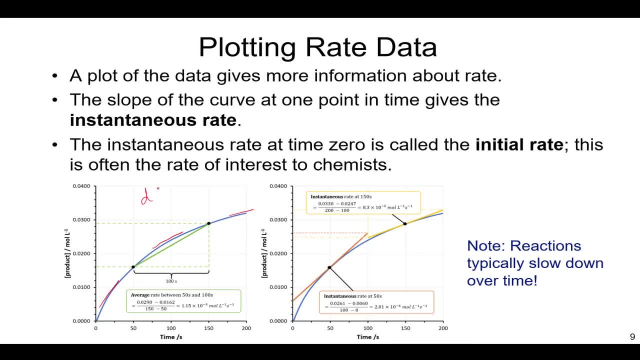 where the calculus comes in, because the slopes of these lines right, db, dt- is really what we're talking about for the rate. that's where the calculus comes in. now we don't have to know the advanced calculus to understand the chemistry that's happening here, but for the more advanced 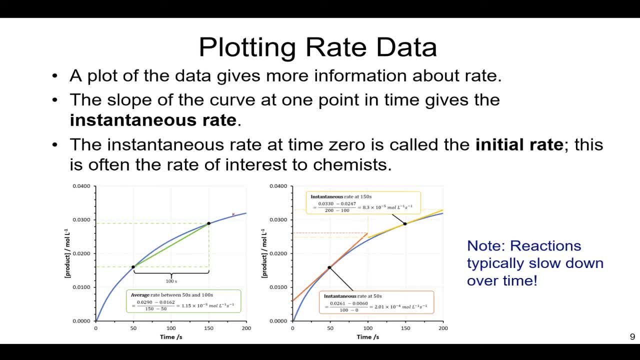 that's really what the rate is talking about. instantaneous rate is the tangent to the slope or the tangent to the line, the slope of the tangent to that line. i should say at that specific point now, this instantaneous rate at time zero, we can look at the point at zero. what is the slope? 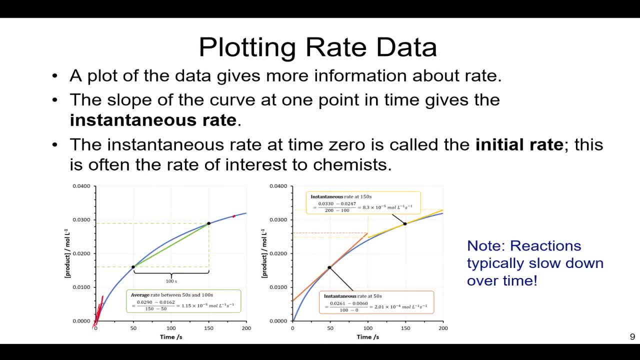 here. well, this slope here is going to be our initial rate okay, and that's often the rate of interest to chemists, because, well, ain't nobody got time to sit around and do reactions for hours and hours. so a lot of times we will mix up reactants in simple proportions. study the 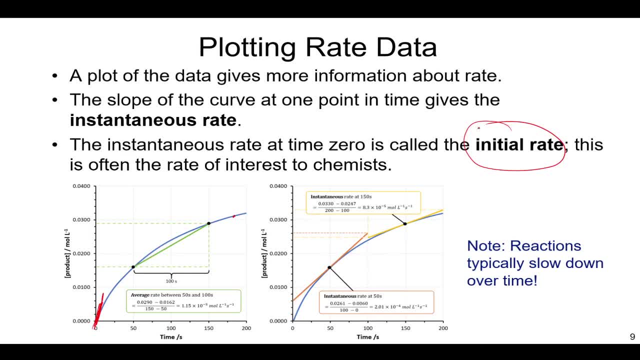 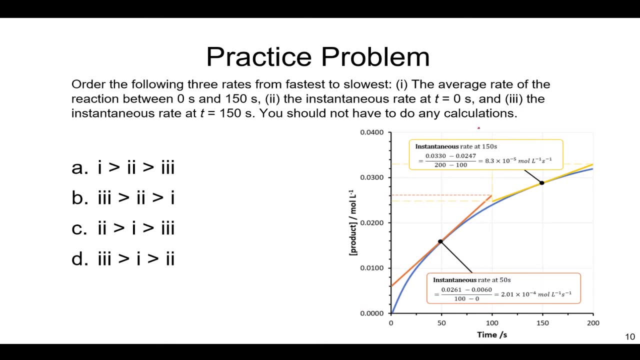 instantaneous rate. then we'll change the concentrations of our mixture, run another reaction and study the rate and we'll see how this gets into the math of telling us something about the rate law in future videos and lectures. now, with all this in mind, let's take some time to do. 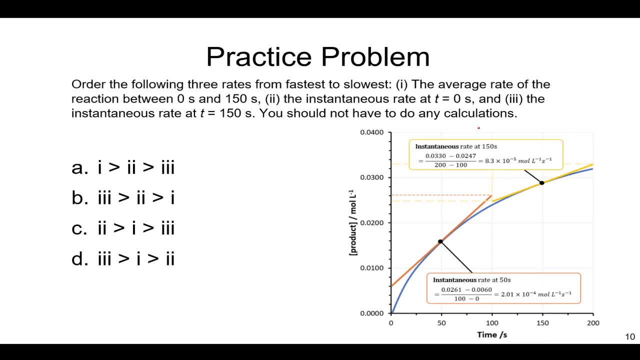 this some practice problems. so here's a practice problem. if you're watching this video, feel free to pause now and work it out on your own, otherwise i'm going to proceed and solve it. order the following three rates from fastest to slowest: one: the average rate of the reaction between zero and 150. two: the instantaneous rate at time. 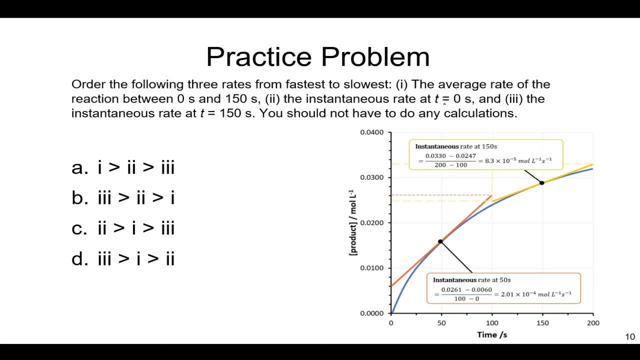 equals zero three. the instantaneous rate at t equals 150 seconds. note: you should not have to do it at the same time. you should do it at the same time. you should do it at the same time. any calculations? okay. so what we're trying to do here is order these three rates, because we 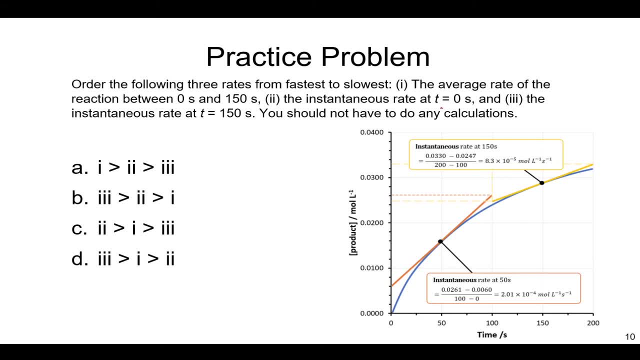 know the rate of the reaction changes over time. order these three rates from fastest to slowest. so the average rate of zero to 150 would be basically the slope of the line from this point to this point. okay, that is the average rate. it's a roughly straight line. uh, the slope from zero to 150. now we can look at the instantaneous. 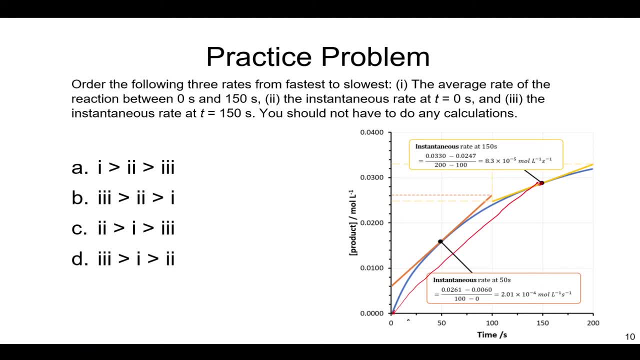 rate at time equals zero, perhaps choosing another color, and that is the slope here. so that's two: red is our one and green will be our three, where green is the instantaneous rate at 150. that's kind of shown here already with this orange line, but i'll redraw it again. 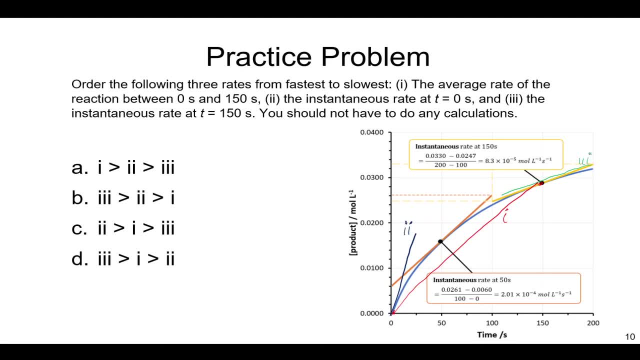 there we go, that's three. okay, so the steeper it is, the faster it is so clearly here, the fastest is going to be our instantaneous rate at time zero. the average is not going to be the next steepest and the least steep is going to be three, so it should be two, one, three. it should be this guy right here. 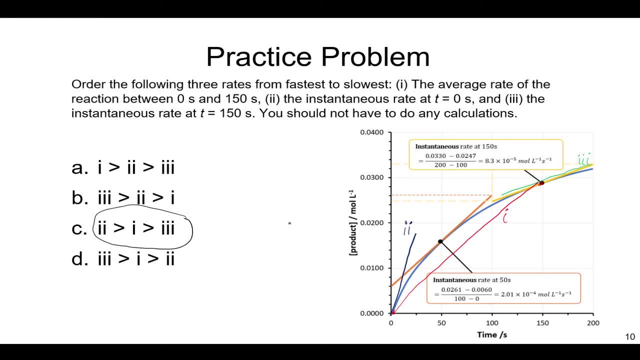 and again. that makes sense because the rate should slow down over time. so the instantaneous rate at the initial should be the fastest, the instantaneous rate at the end should be the lowest and the average obviously should be in the middle. Okay, so the correct answer here should be: 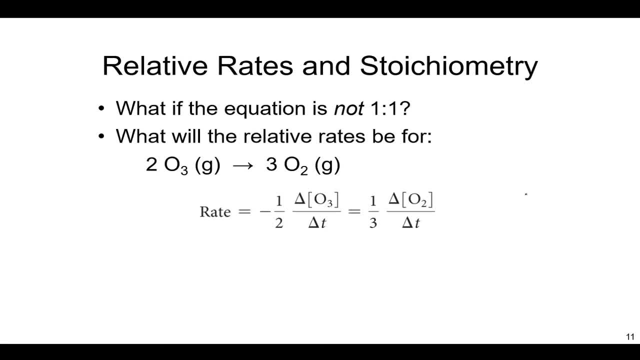 C. Now, not always is it going to be something as simple as A goes to B. A lot of times in chemistry we have coefficients out front. 2A goes to B, And again, this does not necessarily mean that an A has to collide with an A to make B. That is just what happens in the overall process. 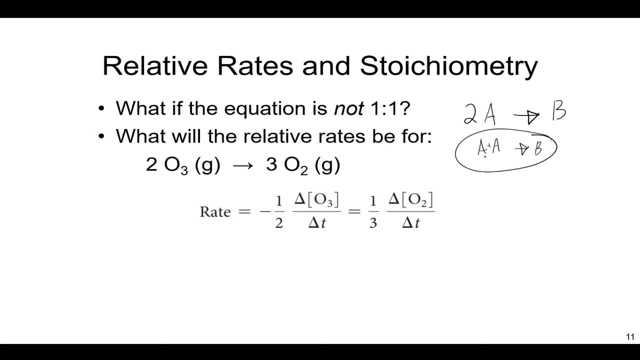 The mechanism is what we're trying to slowly build up to: to figure out exactly what happens on the molecular scale, to make that B Okay. just from the overall reaction you can't write the mechanism of how things collide. That's a very confusing and often missed point. But we're not. 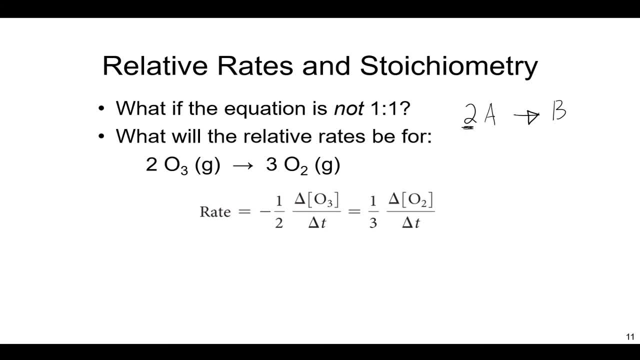 quite there yet, But let's worry about these coefficients for now. And how do they mathematically represent or relate to the rates of products and reactants? We only have to measure one of these things- production of B, to get the rate. 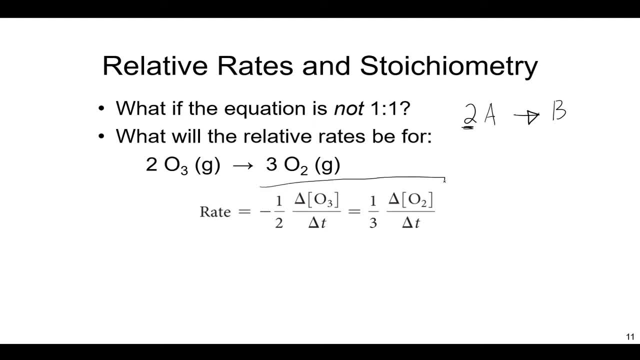 Okay, But we can always relate that to the reactant. Here's an example of ozone turning into oxygen, And this is actually a really important reaction in the atmosphere for controlling the amount of ozone they can get together and make oxygen. We really need this. 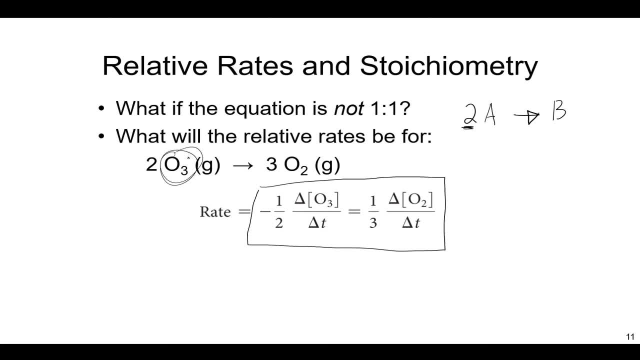 ozone layer to protect us from some of the sun's harmful UV rays. So we don't want to encourage this reaction. if we can help it In any case, we could just measure the concentration of oxygen and get the rate for this reaction. So we can get the rate for this reaction And then we can. 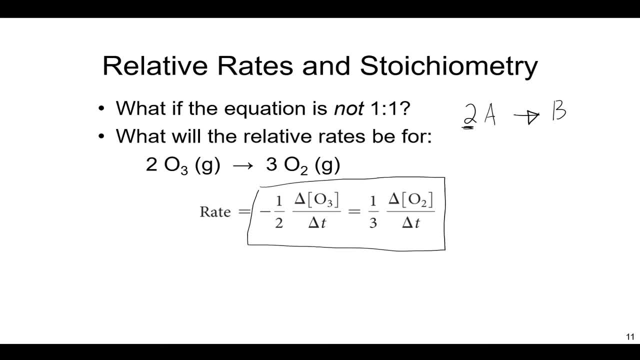 get the rate for this reaction And know, of course, stoichiometrically it should be related to the disappearance of ozone And that's what's shown here. So, like we usually will write a rate is the change in concentration of the reactant. 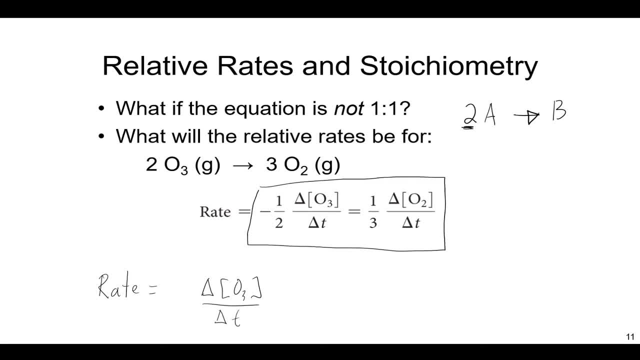 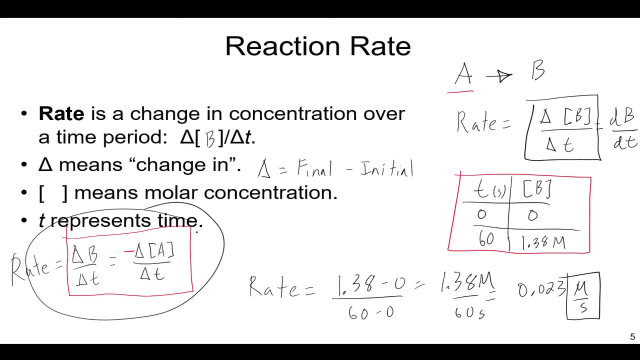 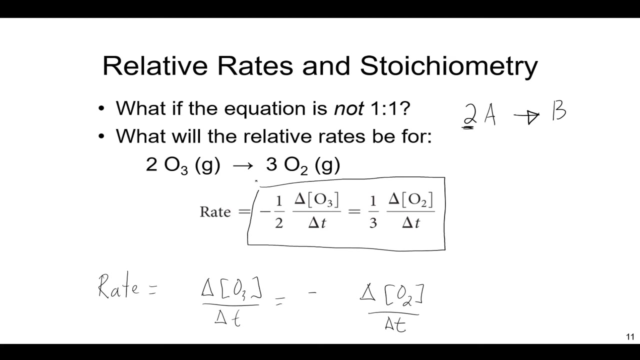 per change in time, or the negative change in product per change in time. But that was really only for these one to one cases. back here, A goes to B. if there's stoichiometry or coefficients involved, well, it's a bit different. We have to divide by that coefficient. Okay, so this ozone that has a. 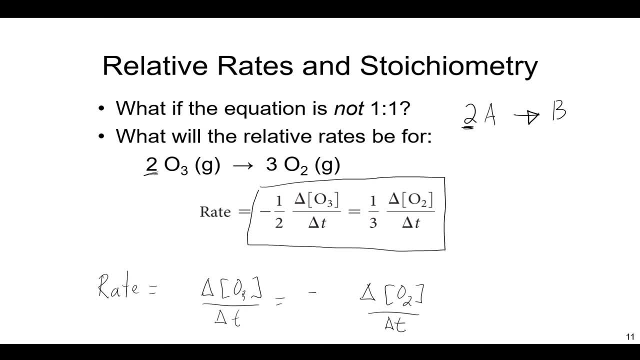 two out front. I'm sorry, I mixed these up. this was supposed to be the product delta O2. And this was supposed to be the reactant O3. That's why there's a negative sign, because for the reactant there should always be a negative sign out front. 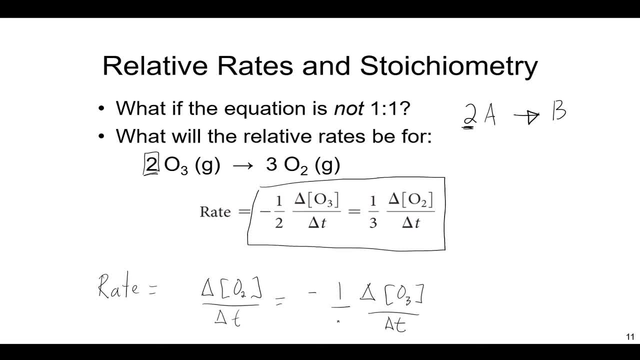 So if there's two ozones, I divide by that, So I put a one half here. If there's three oxygens, I divide by that and I put a one third here. So this now represents the relationship of the rates. 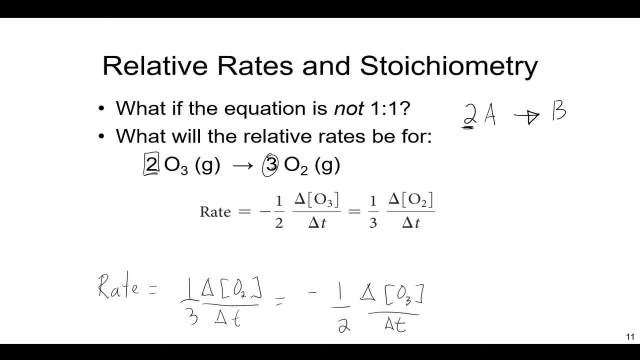 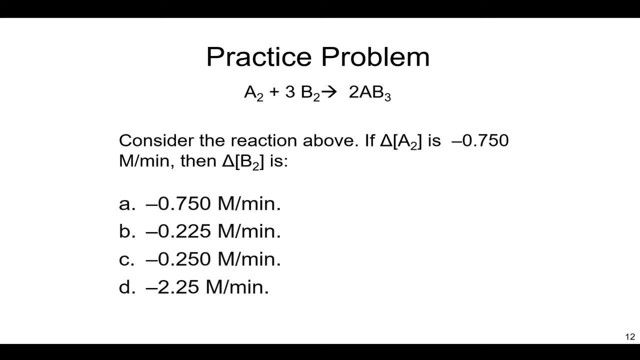 Okay, just showing you how to include stoichiometric coefficients here. So let's look at this in practice and try another practice problem. Consider this reaction above And here I'll give you the change in concentration of A in molarity per minute. So that's actually a rate. 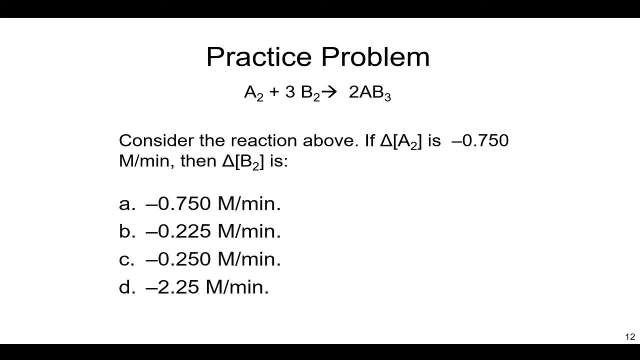 What is the change in concentration of B? Pause the video now and try, before I proceed, and solve it Just from the stoichiometry. okay, we can write: the rate is negative, change of A2 per change in time And that's going to be equal to a positive. 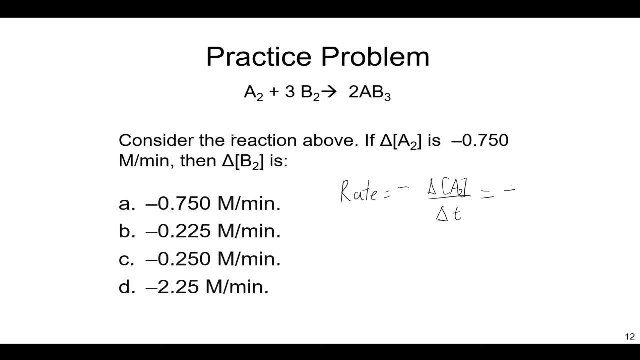 Sorry, negative. No, it's still a reactant. The negative of delta B2.. Delta T: but this has a coefficient of three here, So this should really be negative one third. So if this delta A2, delta T is negative, point 750.. 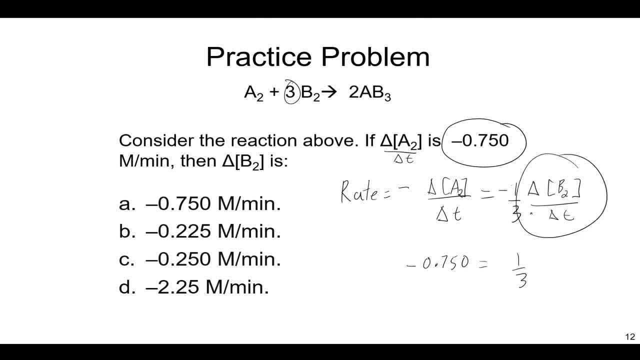 That is one third of this value. And the negative signs? well, these will just cancel out effectively. So negative point 750 equals one third of delta B2.. Delta T: They'll multiply both sides by three And there's our result. 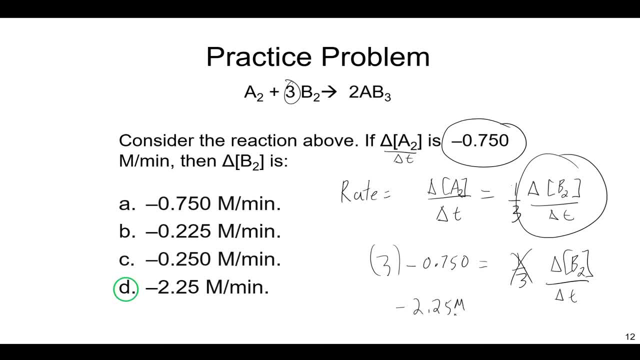 Two point, sorry, negative 2.25 molarity per minute. So we have a negative one third of delta B2.. So it's going to be negative one third of delta B2.. Okay, so these are sort of the basics for calculating these rate constants and relating the stoichiometry from reactants to products, right? 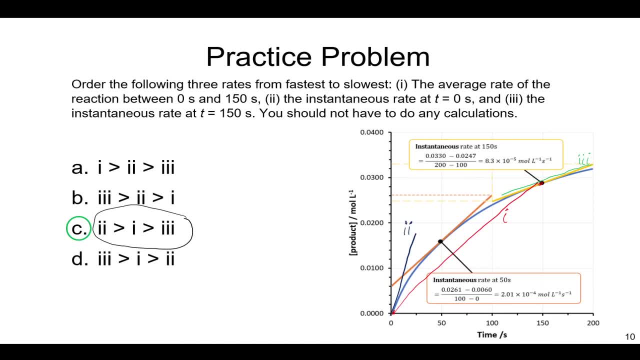 How graphically they look when we plot out the data. In the future lectures we're going to see how doing experiments like this tells us something about the molecular level details of how the reaction actually occurs. right, This reaction mechanism that allows us to do this. 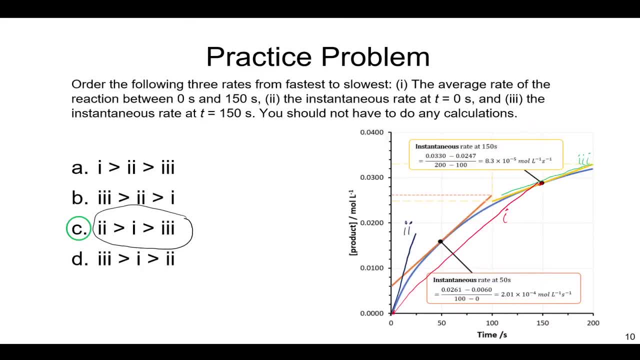 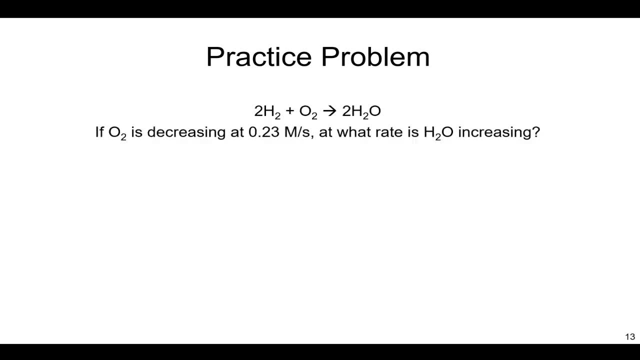 That, ultimately, is what we're after in kinetics, but it takes a while to build up to that point- understanding all this math and the relationships- to be able to actually move forward and do something beneficial. Now we can try one more practice problem before we end here. 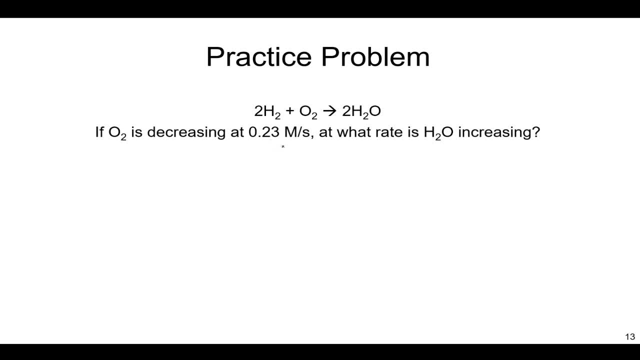 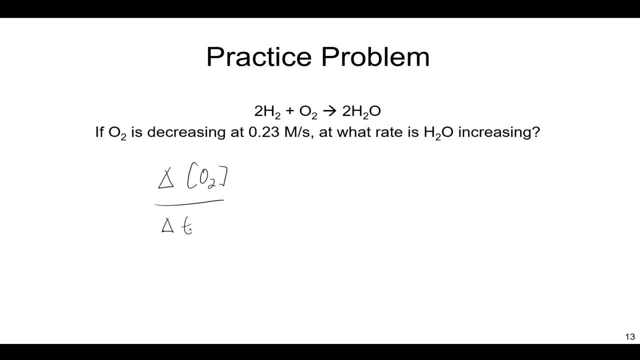 If you would like, Delta, O2, delta T, This rate- That's a reactant, so negative- is going to equal positive Delta H2O, Delta T, This two and water becomes a one half out here, And so if O2 is decreasing at point two, three molarity per second, that means negative. 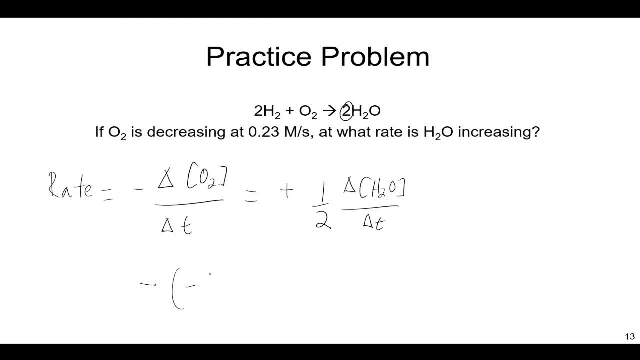